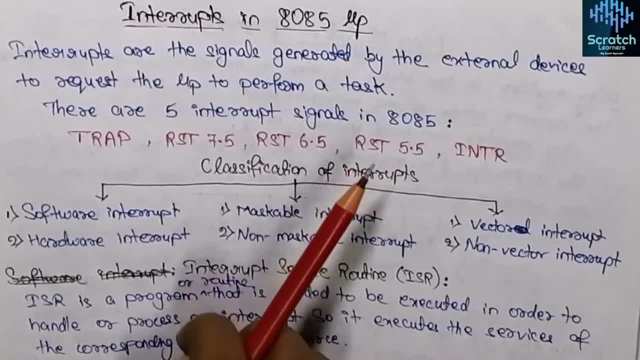 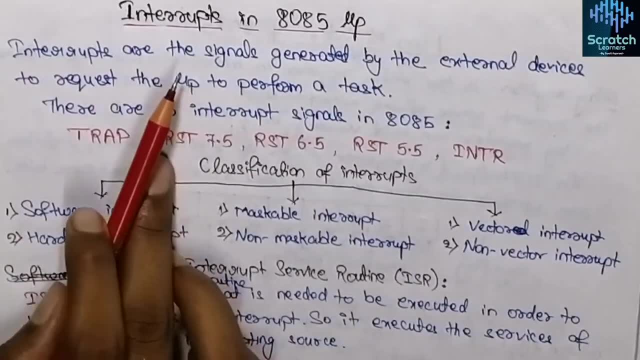 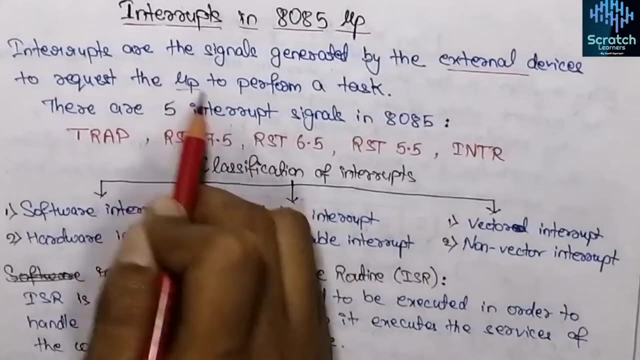 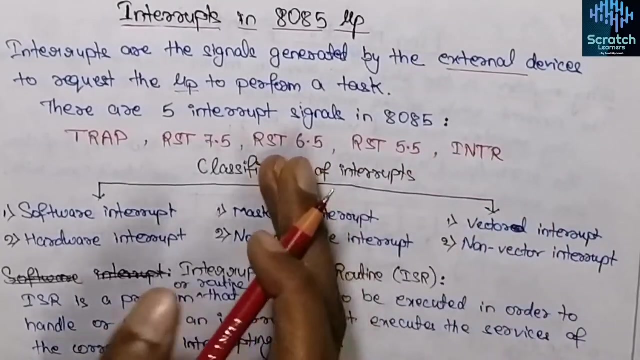 going to discuss about interrupts, what are different types of interrupt signals and the classification of interrupts. so the most basic question: what is interrupts? the interrupts are the signals generated by the external device to request the microprocessor to perform a task. so these are the signals which are generated by some external device. that means 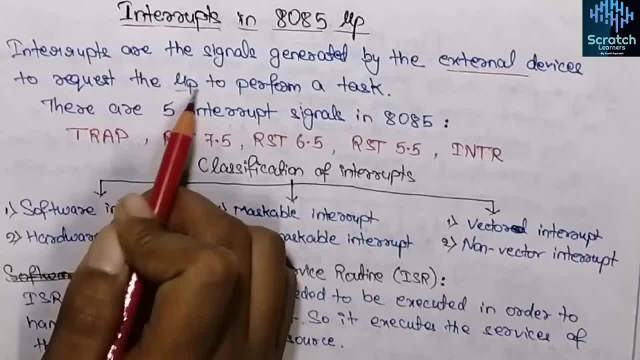 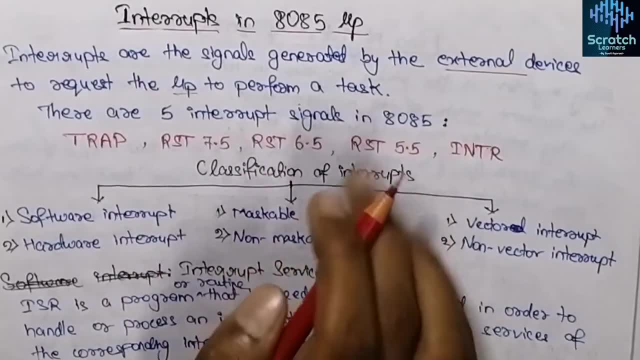 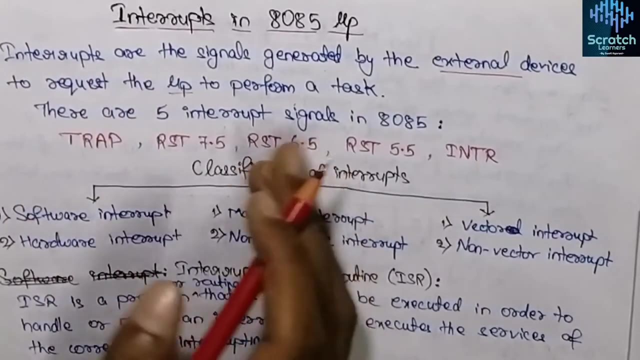 some devices other than the microprocessor to request the microprocessor to perform a specific task. so in a gist we can see that interrupt is a process where external device can get the attention of microprocessor and these interrupts can be initiated at any time without reference to the system clock, so the interrupts can be generated. 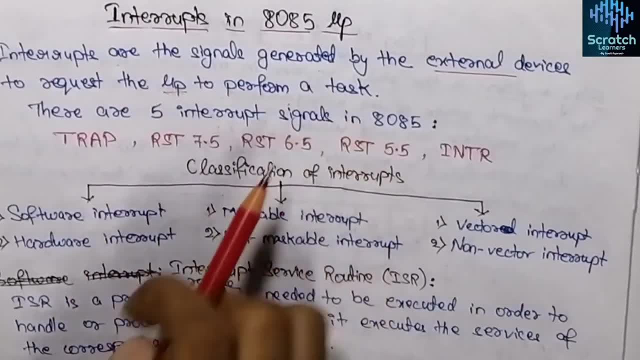 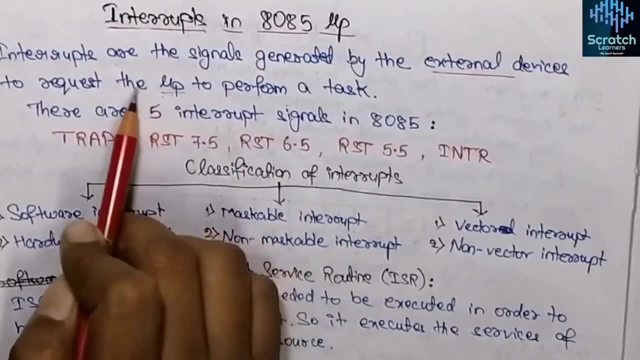 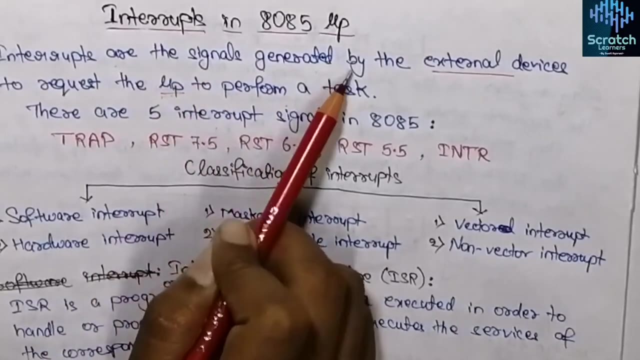 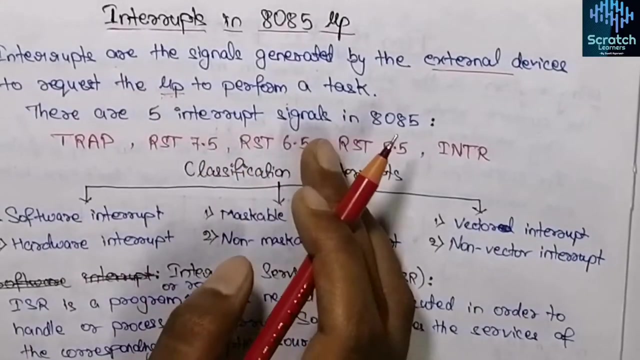 at any time. but the response to an interrupt is directed or controlled by the microprocessor. so how does microprocessor get to know when an interrupt comes and how microprocessor work for that interrupt? so in the beginning the external devices transfers some signals to the microprocessor to respond to some high priority external initiated signals. and when microprocessor 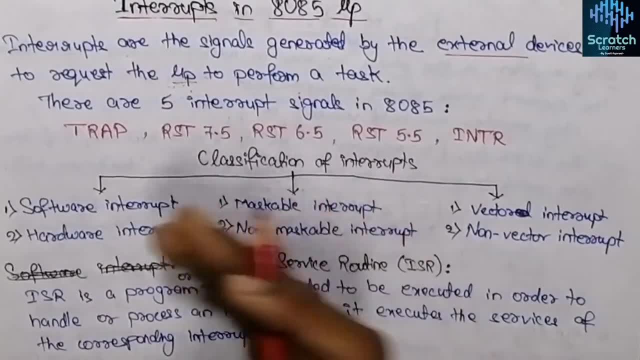 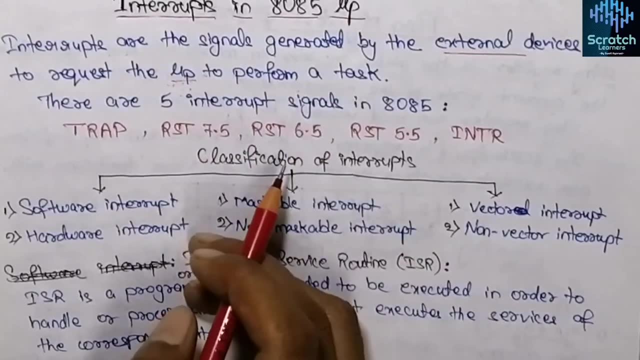 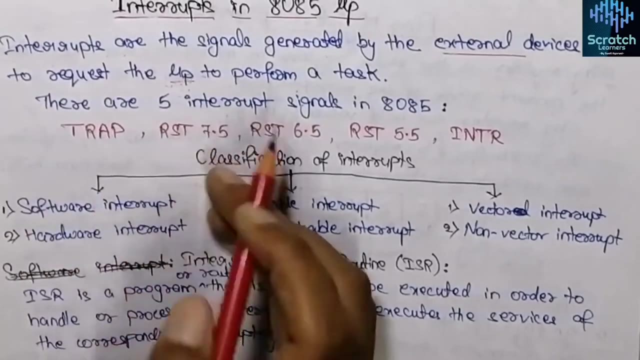 receives an interrupt signal. that means when an interrupt signal is detected by the processor, then the microprocessor suspends the execution of its current program and it start executing the program corresponding to the interrupt signal. so when the microprocessor suspend the currently executing program, then the control will jump. 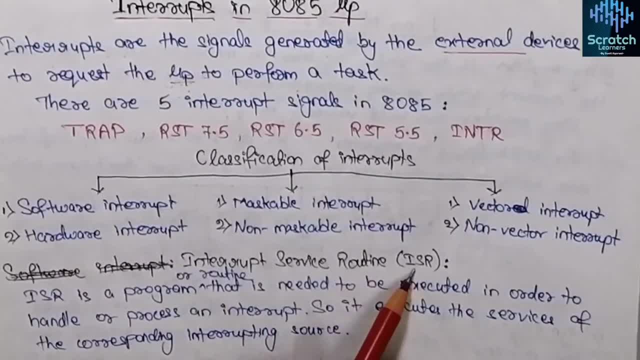 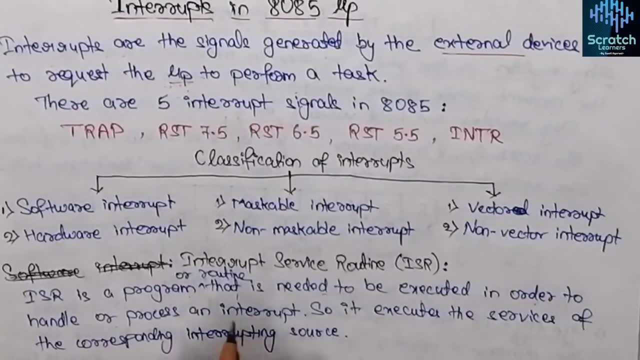 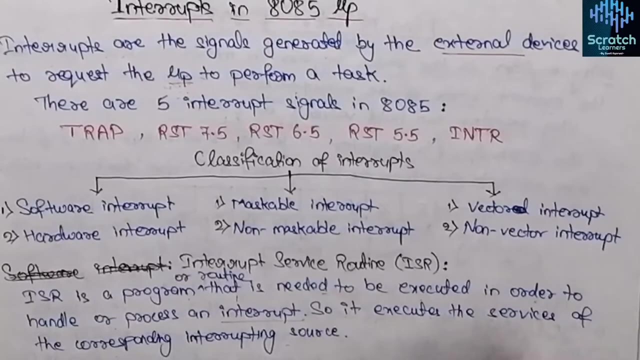 to the isr that means interrupt service routine. what is this? this is a program or routine that is needed to be executed in order to handle or process an interrupt. so this is a main program needed for the execution of interrupt. so it executes the services of the corresponding 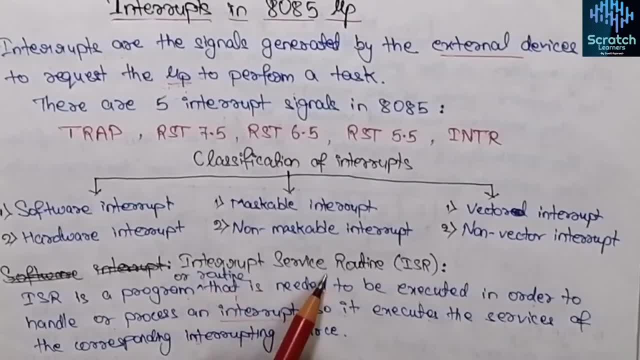 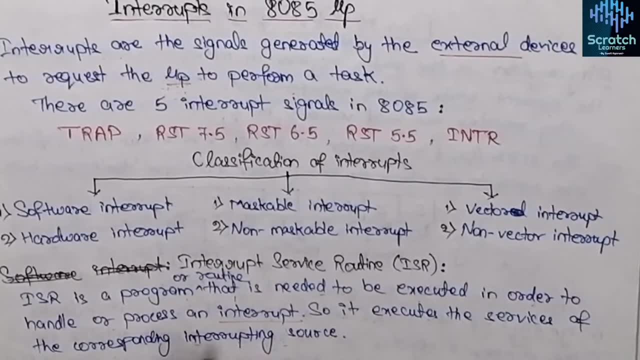 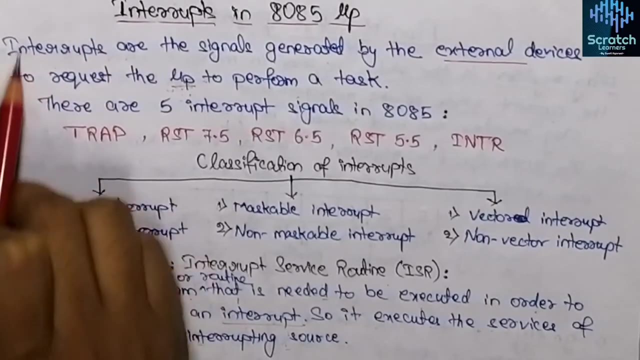 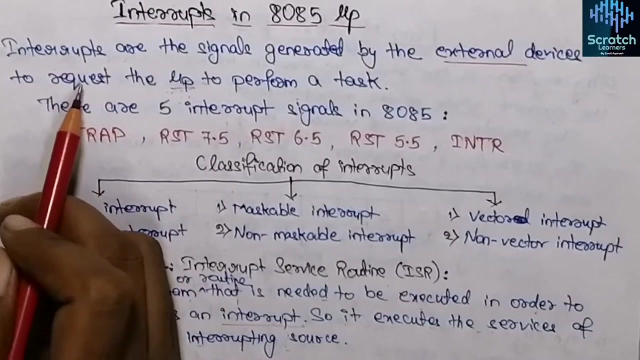 interrupting signal source. that means there is a specific isr for all the corresponding interrupts and for a specific interrupt its corresponding interrupt service routine is being executed. so this was about when an interrupt is being handled and when the process of interrupt handling is done, that means whatever instruction it need to be executed is completed, then the microprocessor again start. 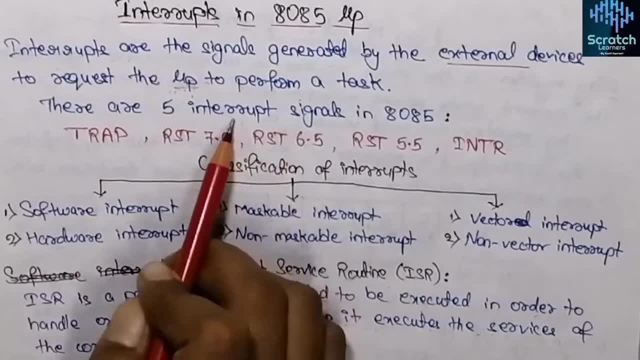 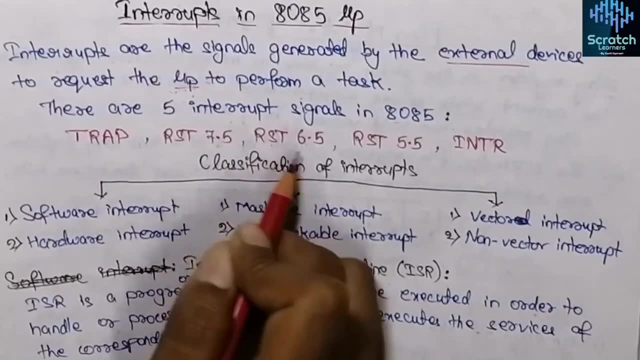 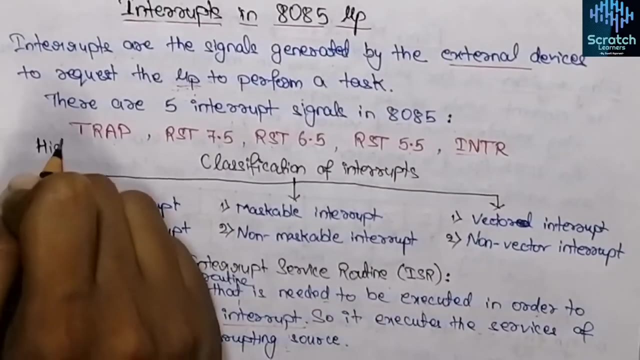 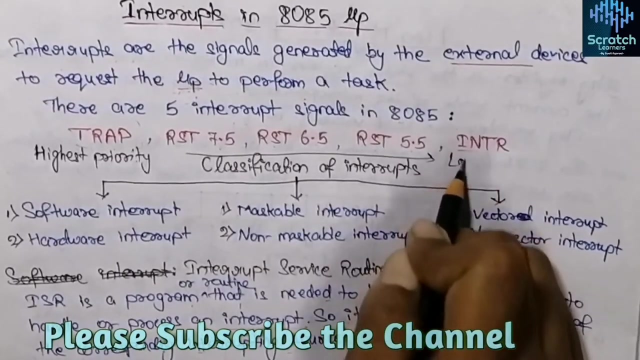 to resume its incomplete task. so there are many interrupts in 8085. so the first one is trap, then rst 7.5, rst 6.5, rst 5.5 and intr. here in these five interrupts the highest priority is for trap- okay, and the lowest priority is for the intr signal. 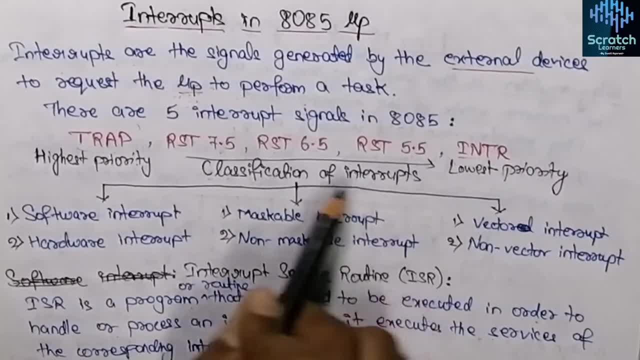 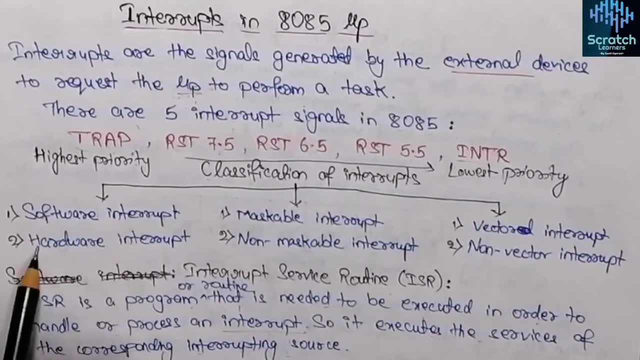 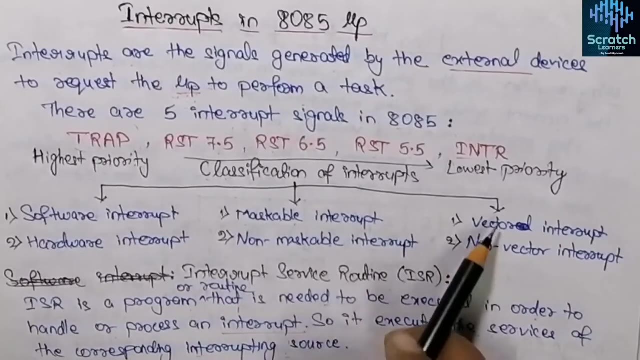 now let's come to the classification of interrupts. so the interrupts in 8085 are can be classified in three ways. the first one is the software interrupt and the hardware interrupt. the second way is the maskable and non-maskable interrupt, and the third one is 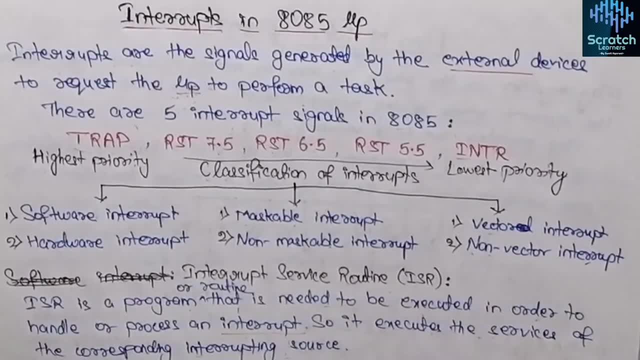 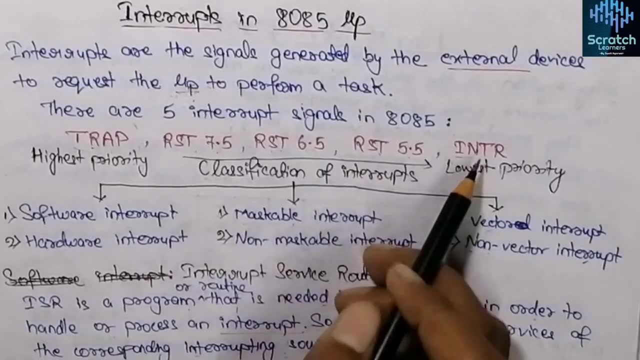 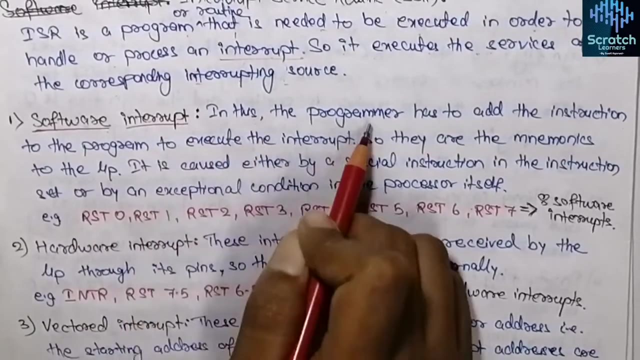 the vector interrupt and non-vector interrupt. so now let's discuss about all these classification of interrupts, and then we will discuss about all these interrupt signals one by one. so here, the first one is the software interrupt. so what is it in software interrupts? the program has to add the instruction to the program to execute the interrupt. so here, 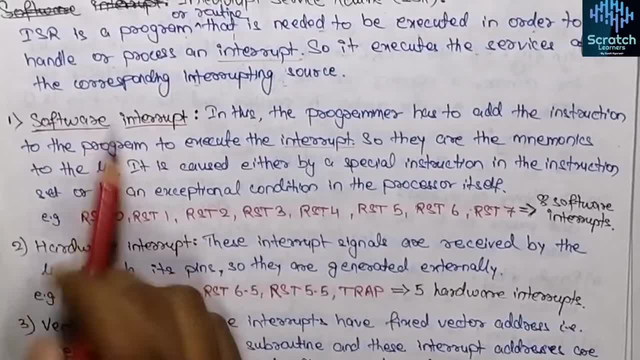 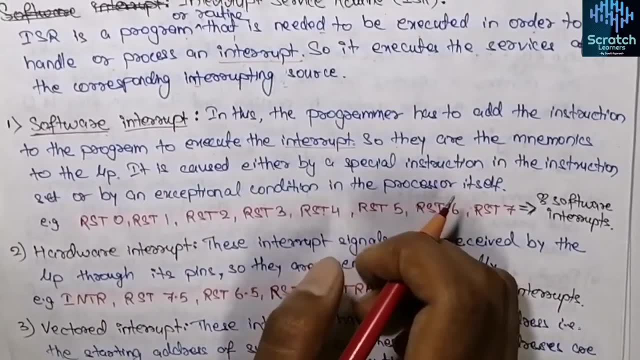 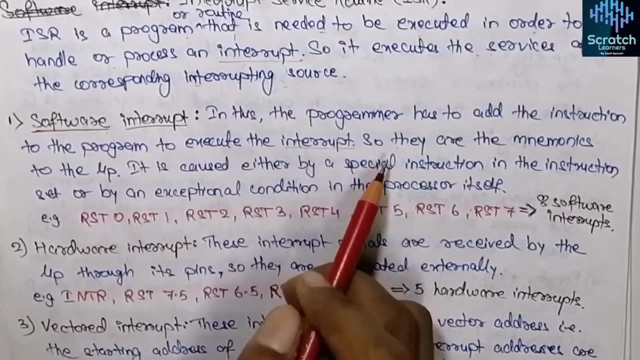 the programmer adds the instruction of the interrupt, so they are the mnemonics to the microprocessor. as we know, the microprocessor works in assembly language program, so mnemonics are used to program right. so the software interrupts are being fed into a program by adding the instruction. that means the mnemonics to. 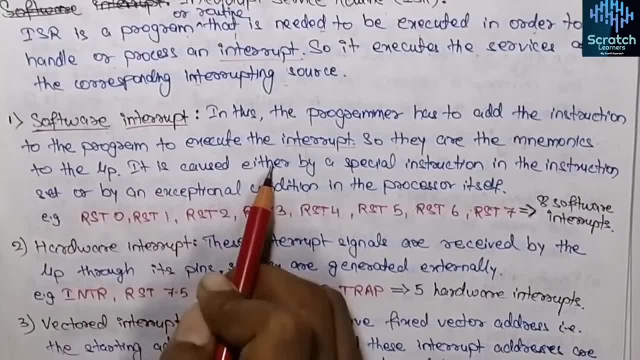 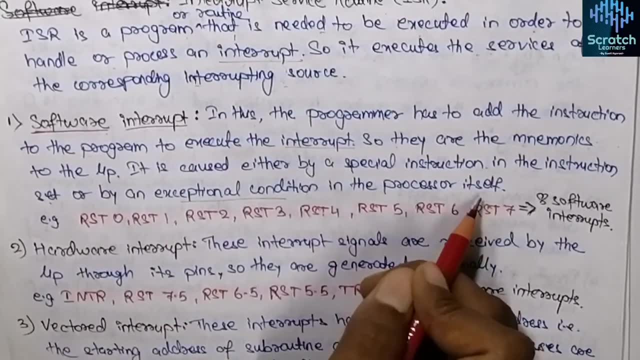 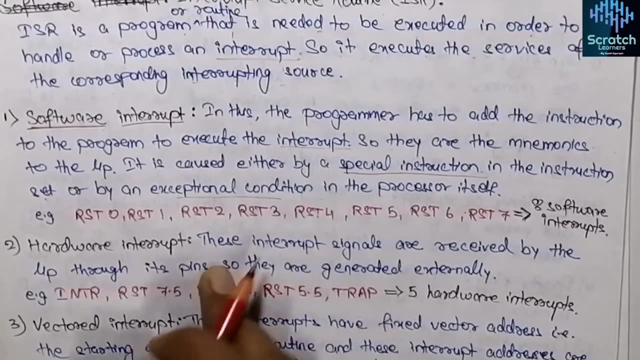 the microprocessor, and the software interrupt is caused either by a special instruction in the instruction set or by an exceptional condition in the processor itself. so these are the main two ways by which a software interrupt can be generated. now what are the software interrupts? in 8085 there are: 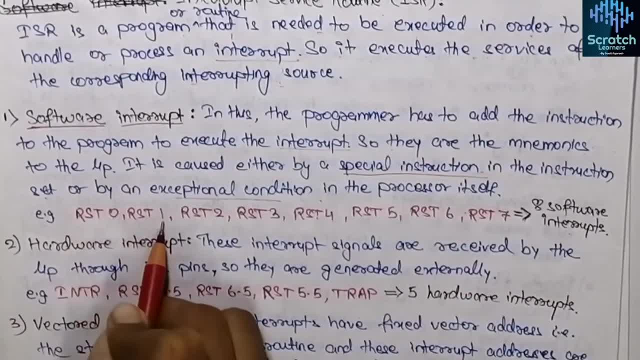 eight software interrupts. they are: RST 0, RST 1, RST 2, RST 3, RST 4, RST 5, RST 7, RST 8, RST 10, RST 11, RST 12, RST. not RST 3, RST 5, RST 8, RST 9, RST 11, RST 10. 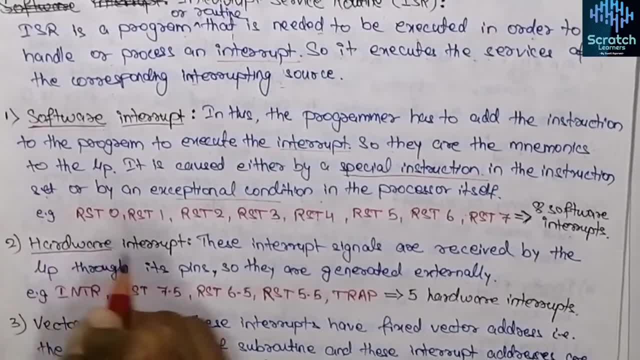 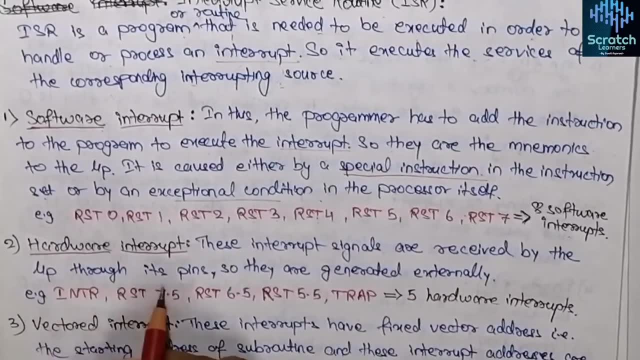 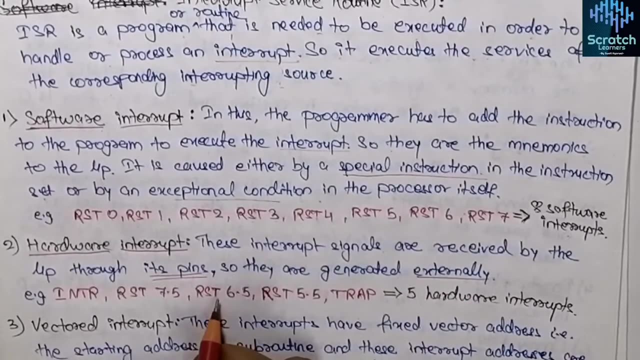 rht6 and rht7. now the next one is the hardware interrupt. so the hardware interrupt are the interrupt signals received by the microprocessor through its pins, so they are generated externally. that means here an external device initiates the hardware interrupt of 8085 by placing an. 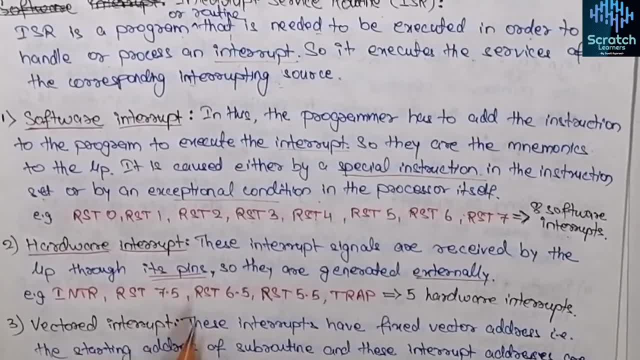 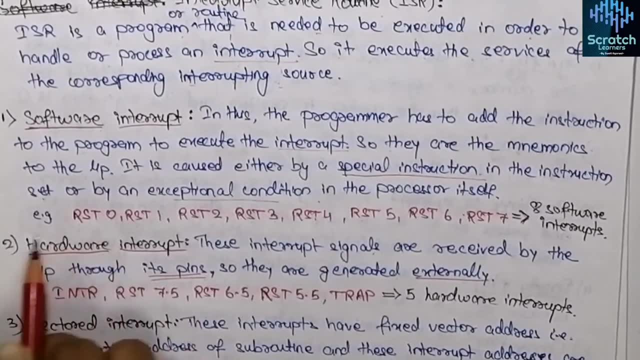 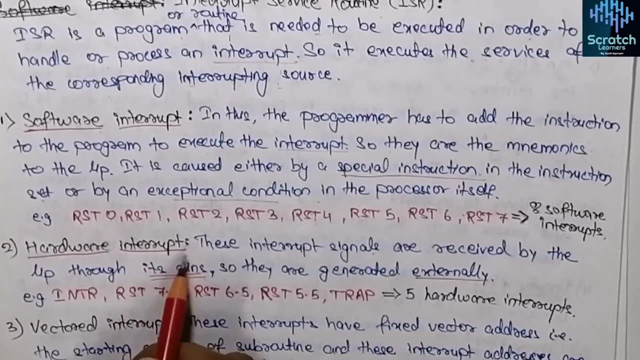 appropriate signal at the interrupt pin of the microprocessor, as the interrupt signals are generated through its pins. that's why it is called a hardware interrupt. and how does the microprocessor comes to know whether a hardware interrupt is occurring or not? the processor keeps on checking the interrupt pins at the execution of the current instruction and if 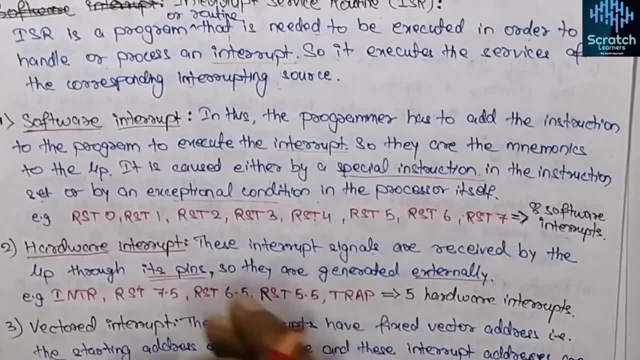 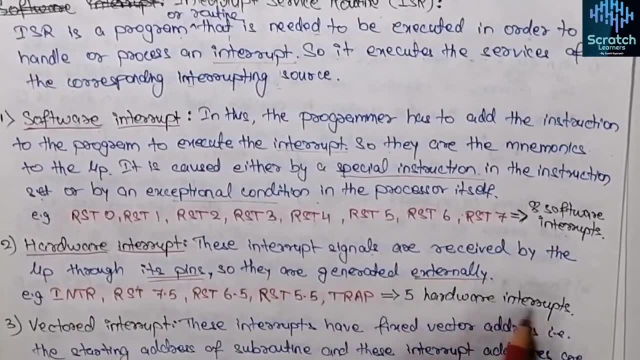 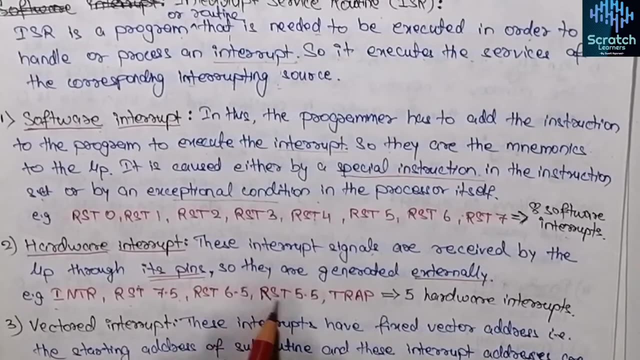 the processor finds a valid interrupt, then the processor accepts that that interrupt. we will discuss about these things later on in this video. and there are five hardware interrupts in 8085. they are intr. rht 7.5, rht 6.5, rht 5.5 and trap. so what is a vector interrupt? 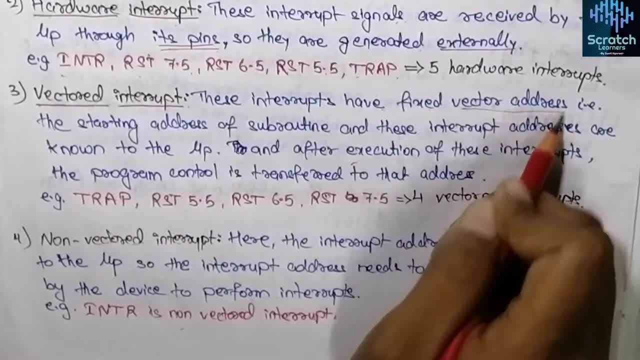 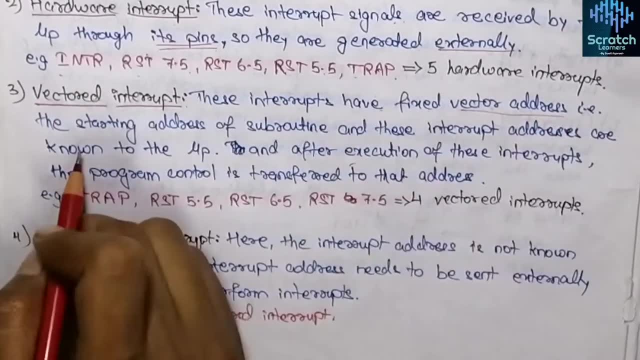 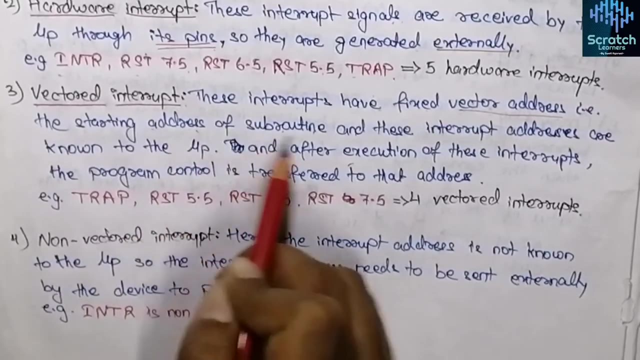 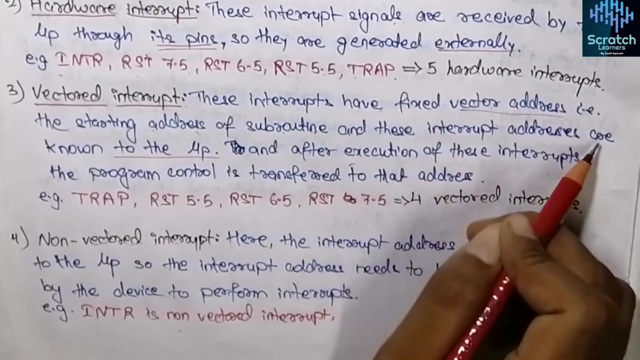 these interrupts have fixed vector address. now here the main term is vector. what is a vector address? vector address means the starting address of subroutine. so the vector address is a specific address from where a subroutine execution will start, and these interrupt addresses are known to microprocessor. this is the main point: that these vector interrupts should be known to the 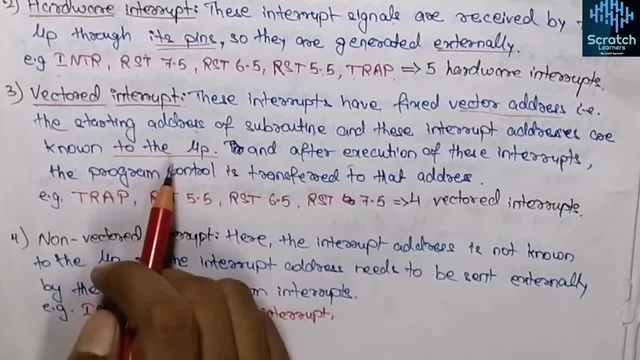 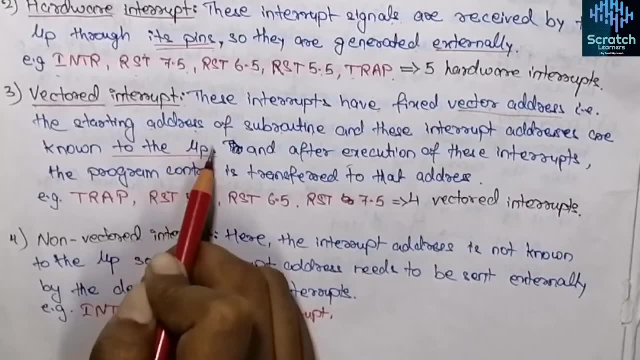 microprocessor that means in vector interrupt. the processor automatically branches to the specific address in response to an interrupt. so the one question that may come in your mind is that how the microprocessor know what is the starting address of the subroutine or what is the vector address where i should map so these 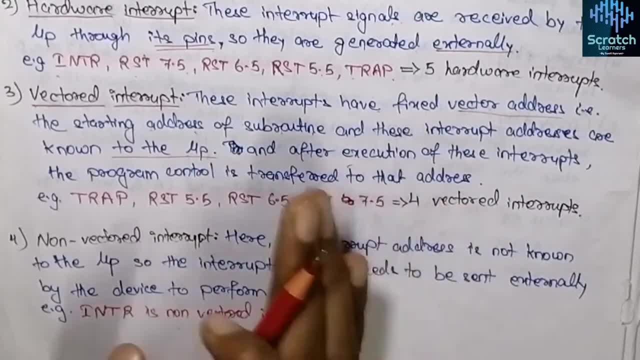 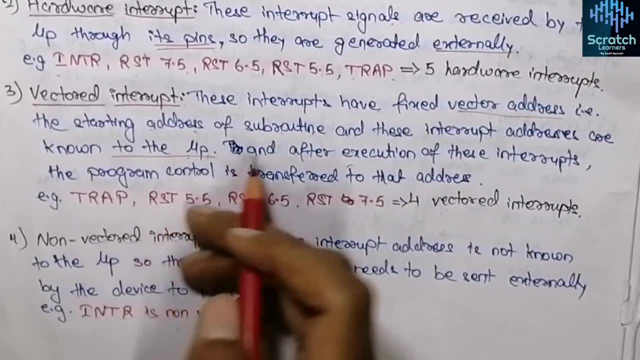 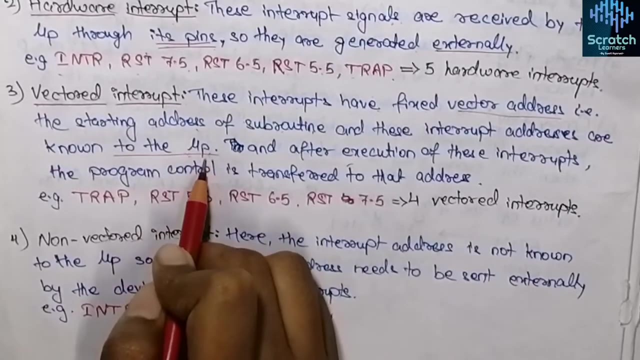 addresses. that means the addresses of isr. we have discussed isr right. that means the interrupt service routine. so the address of the isr, that means the address to which the program control will be transferred, is fixed by the manufacturer so the microprocessor always know what is its vector address. 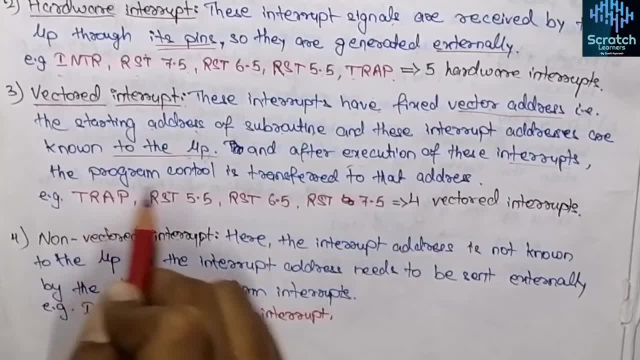 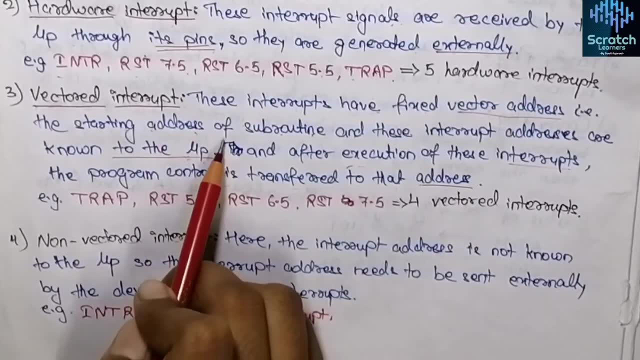 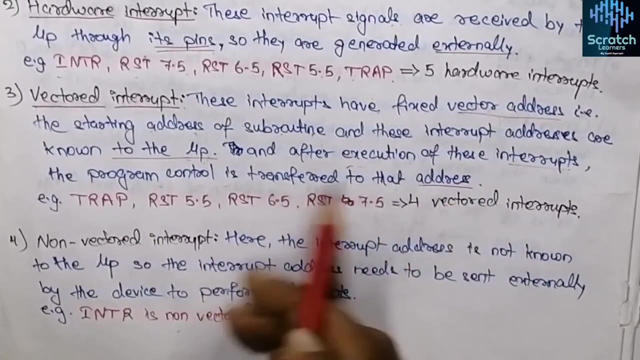 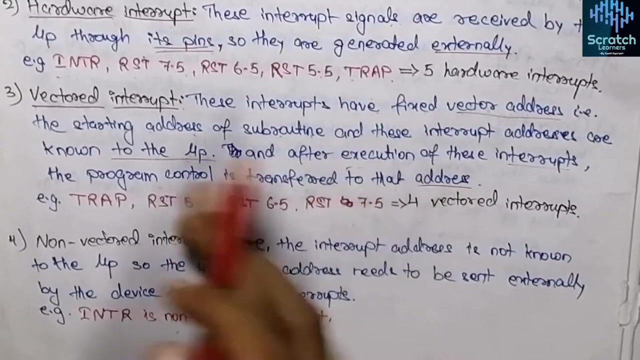 and after the execution of these interrupts, the program control is transferred to that address. so when the microprocessor executes the instruction of that subroutine, then after execution the program control- that means the control of the microprocessor- is transferred to that address. that means the address where the control of the microprocessor was present previously. so there are. 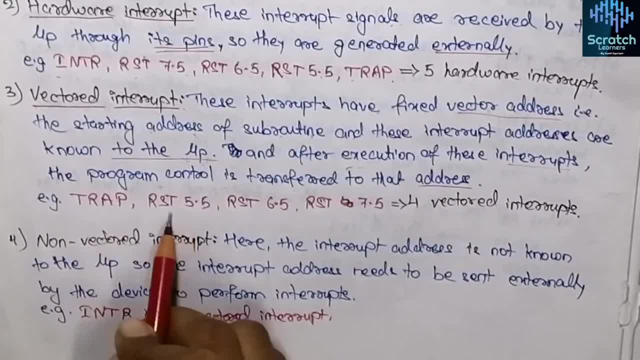 four vectored interrupt in 8085. they are trapped and the other four vectored interrupts are trapped. so the one question that may come in your mind is that how the microprocessor know what is the starting address of the subroutine or what is the starting address of the microprocessor. 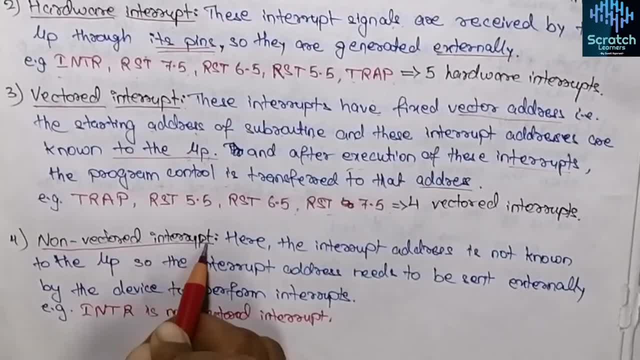 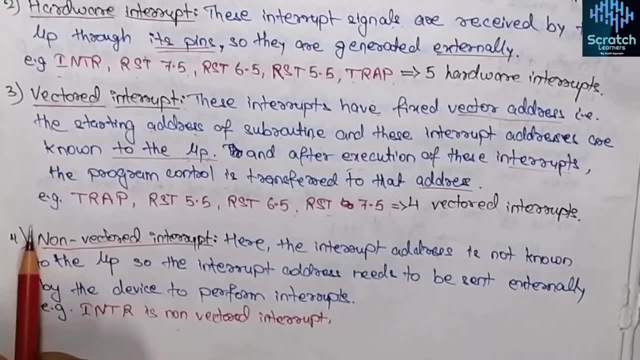 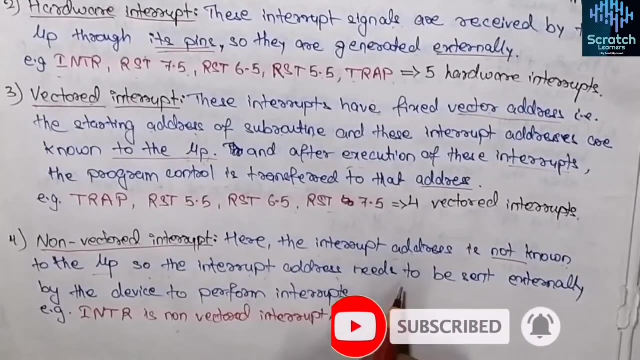 now, what is the non-vectored interrupt? so, as the name suggests, this is the vectored one, right. so here the microprocessor knows the address, but here it is known vectored, that that means here the interrupt address is not known to the microprocessor. the interrupt address. 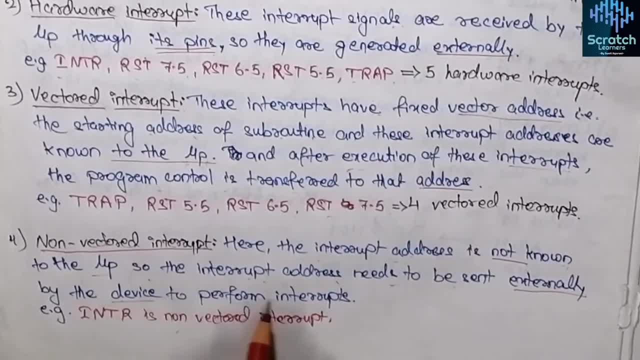 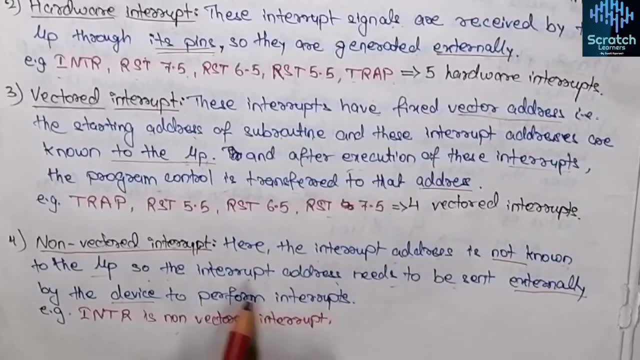 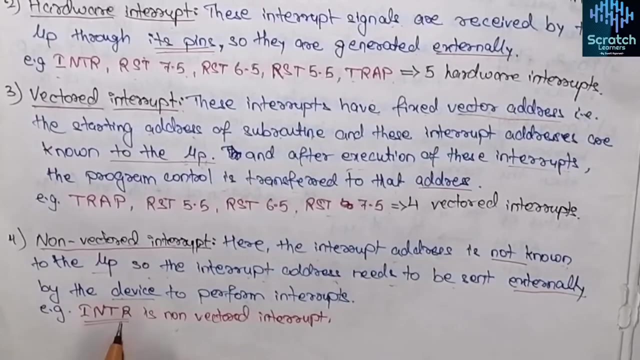 needs to be sent externally by the device to perform the interrupts. this is quite a normal thing. when microprocessor does not know its vectored address, then that interrupt address needs to be sent externally by some device. okay, and intr is the only interrupt that is non-vectored. so here, 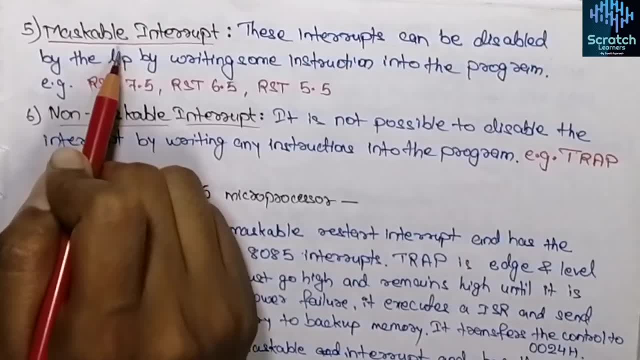 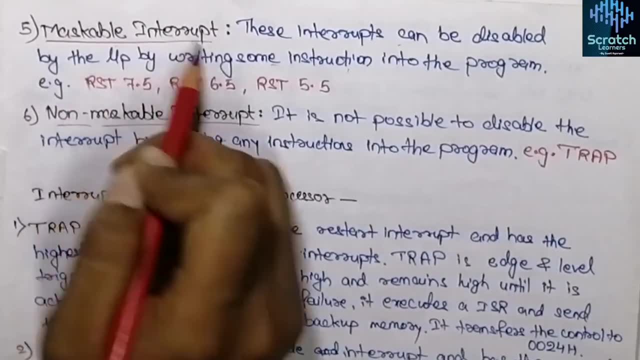 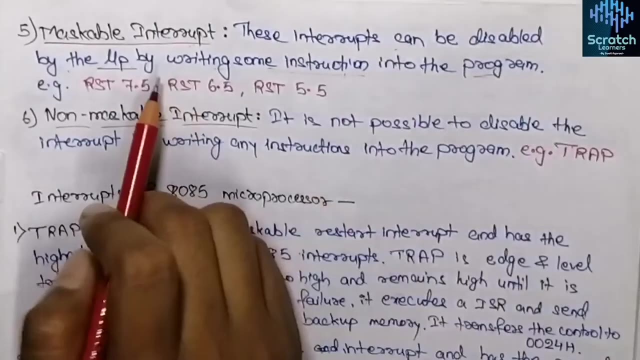 the main term is masking. what is masking? masking is the method of preventing the interrupt from disturbing the main program. so the maskable interrupts are those interrupts which can be disabled by the microprocessor by writing something like this: so the interruption is not known to the microprocessor, so the microprocessor has to send some instruction into the program. and when an 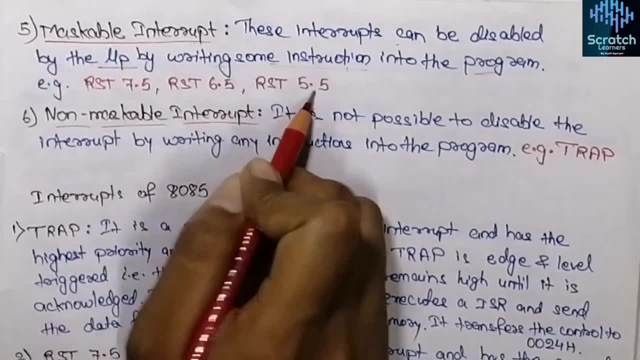 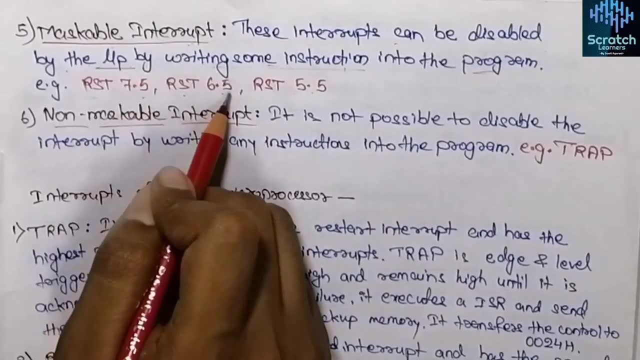 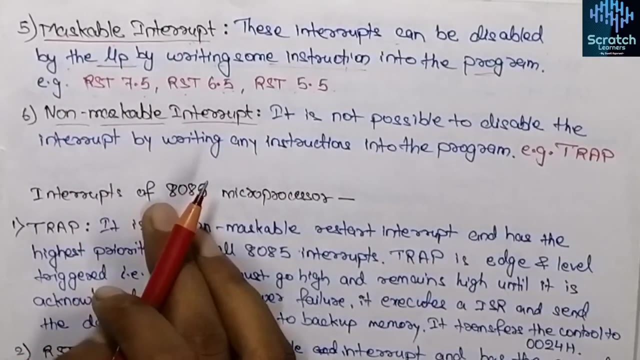 interrupt is masked, then the processor will not accept the interrupt signal. there are three types of maskable interrupts: rht 7.5, rht 6.5 and rht 5.5. these are the maskable interrupts. so what are the non-maskable inter? that? these are just opposite of maskable interrupts. that means it is not possible. 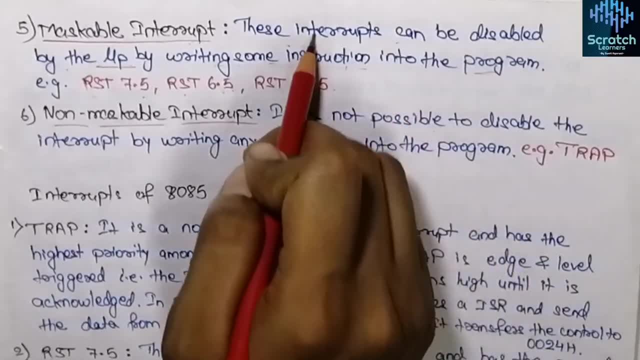 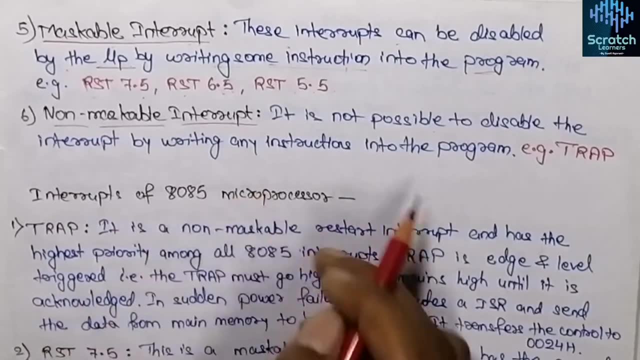 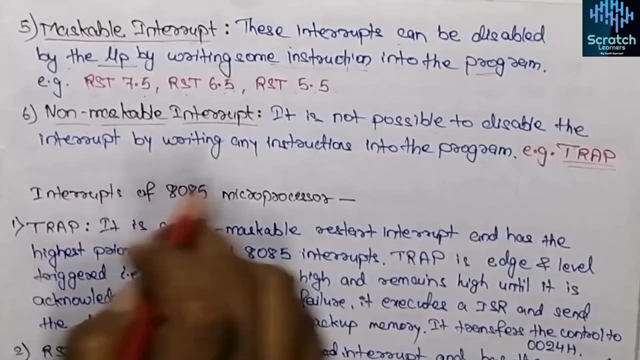 to disable the interrupt. by writing any instruction into the program it was possible to disable the interrupt, but here it is not possible to disable the interrupt. that is the basic difference and the trap is the one and the only non-maskable interrupt in 8085. so this was all about the classification of interrupts in 8085. 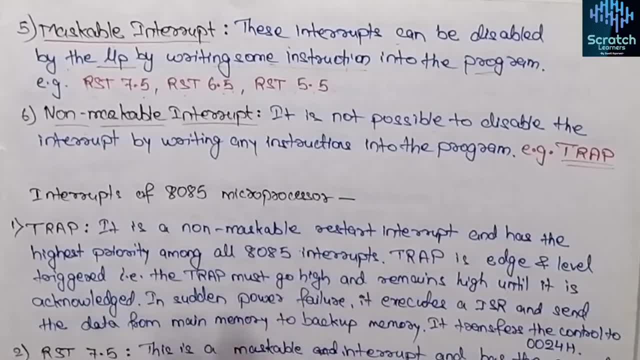 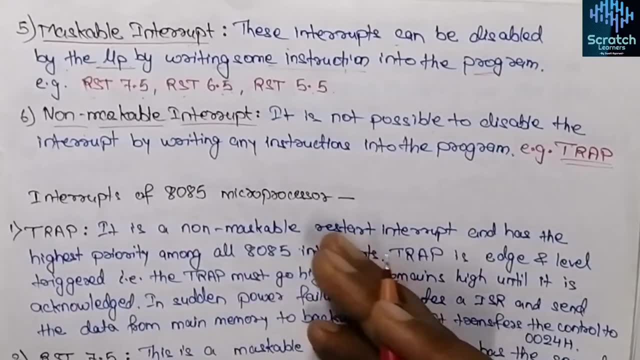 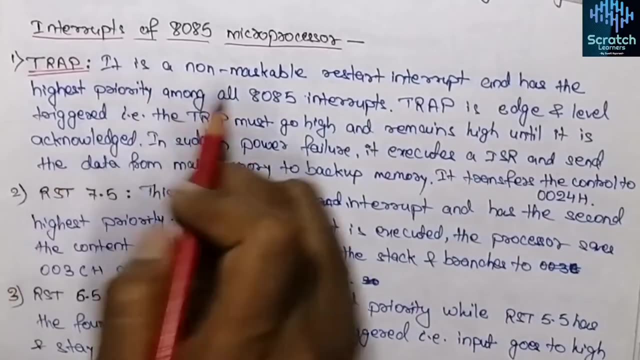 now let's discuss about the interrupt signals in 8085 macro processor. so here we will discuss about trap, RST 7.5, RST 6.5, RST 5.5 and INTR. so the first one is the trap. so trap is a non-maskable. 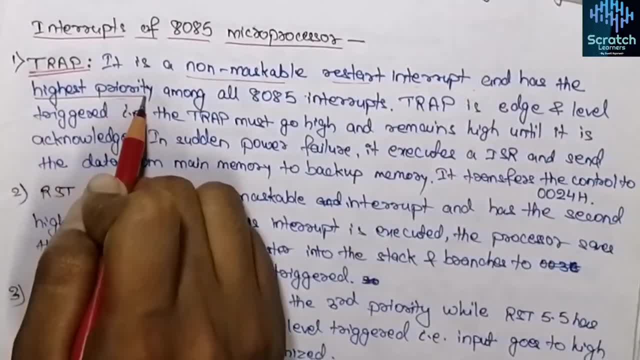 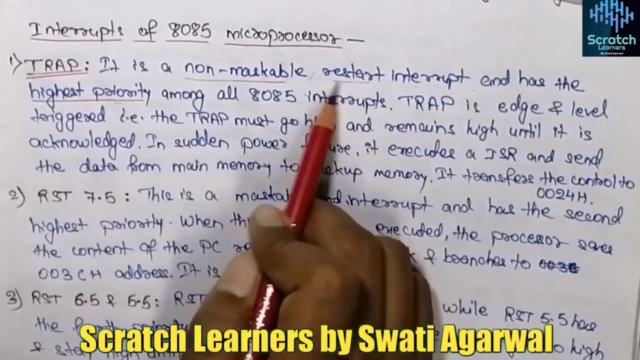 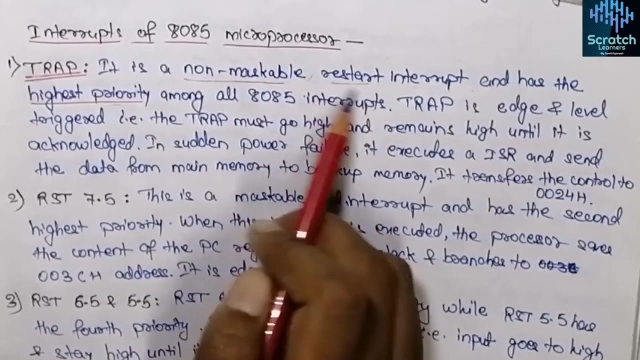 restart interrupt and has the highest priority among all 8085 interrupts. so this is non-maskable- we have just seen now- and restart interrupt. it means that the trap interrupts can only be masked by resetting the mac processor. so that means the restarting the interrupt. that's why it is called restart interrupt. 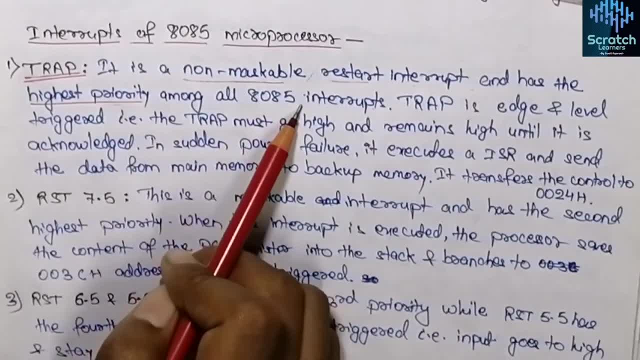 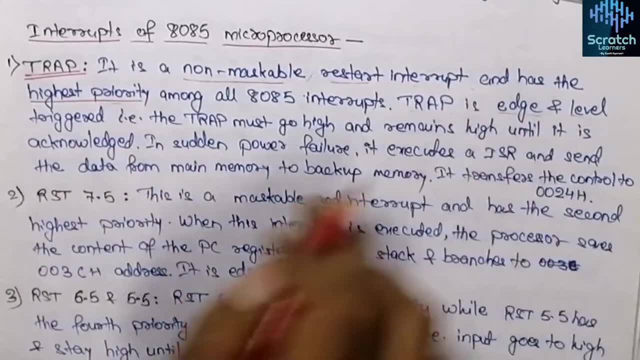 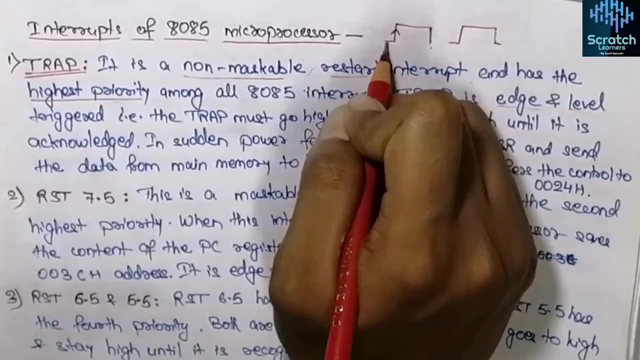 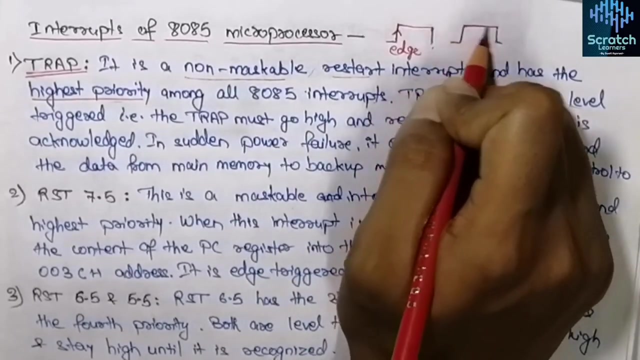 and it has the highest priority among all 8085 interrupts. now, trap is edge and level triggered. what is age and level triggered? see if this be a signal and the triggering is done through edge. okay, this is edge. so this is edge triggering. and in a signal, when triggering is done in level. 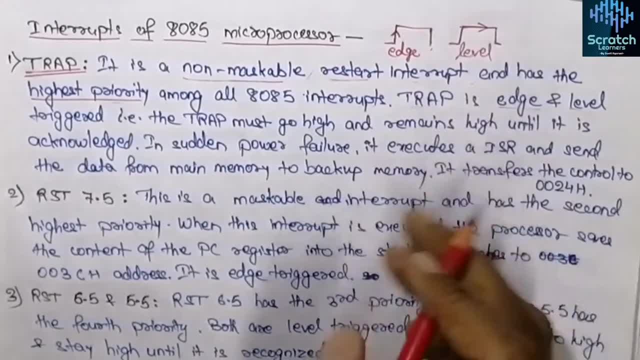 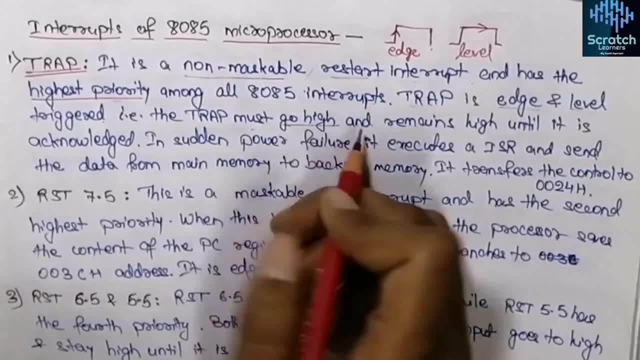 that means the level is triggered. and in a signal, when triggering is done in level, that means this position, then this is level triggering. so trap is edge and level triggered both. that means the trap must go high and remains high until it is acknowledged as trap is edge and 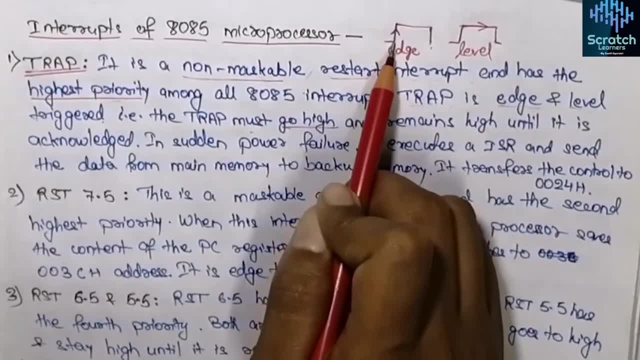 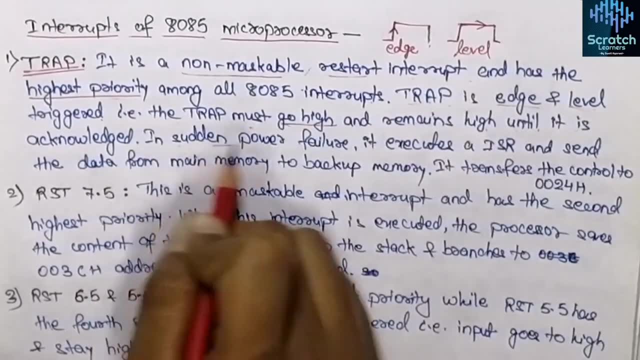 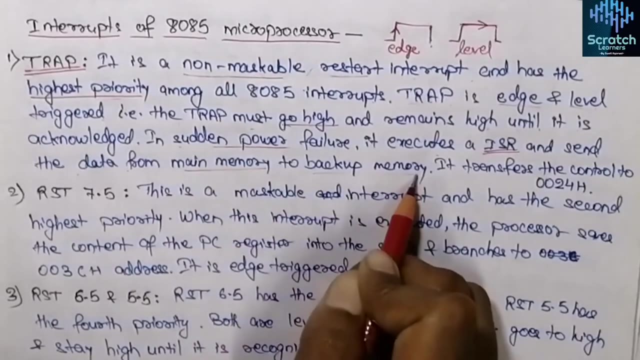 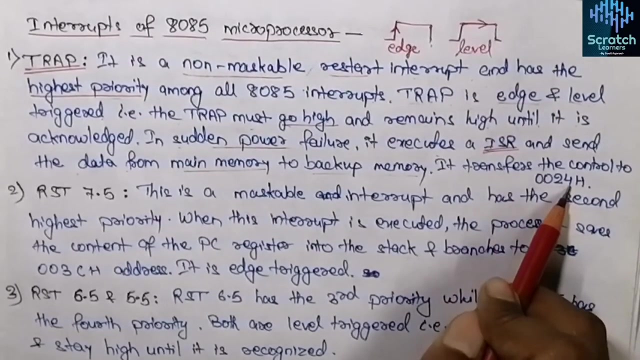 level triggered. the trap must go high here. it will go high and it will remain high until it is acknowledged and in case of sudden power failure, it executes a isr and sends the data from main memory to backup memory and it transfers the control to 0024 hex. that means this: 0024 hex. 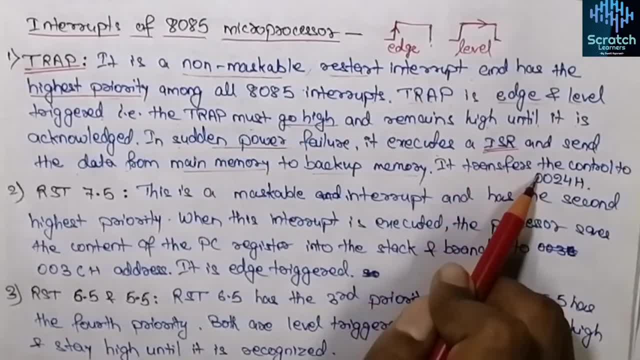 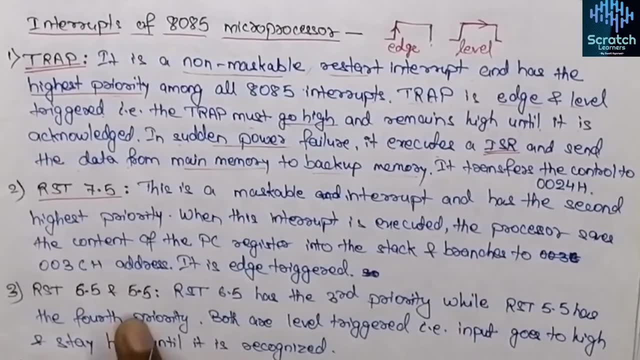 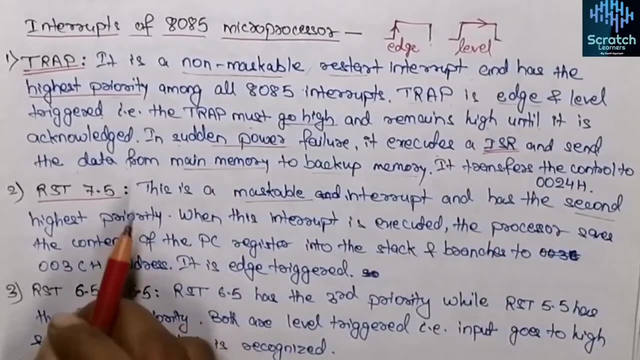 is the address where the program counter will go when sudden power failure occurs. now the next one is the rst 7.5. so this rst 7.5 is a maskable interrupt and has the second highest priority among all the 8085 interrupts. when this. 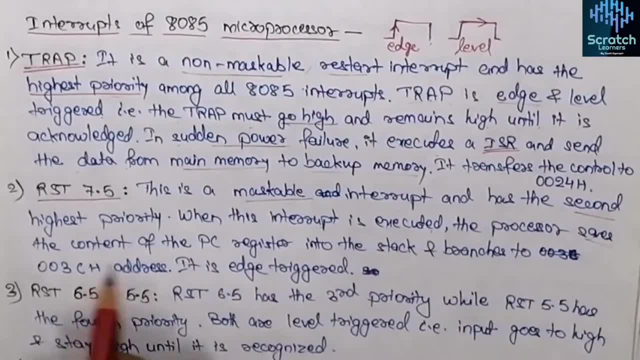 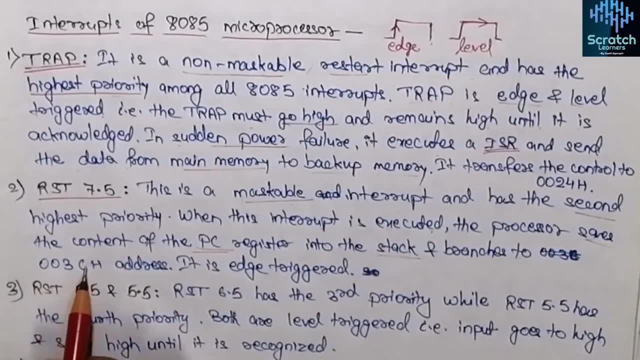 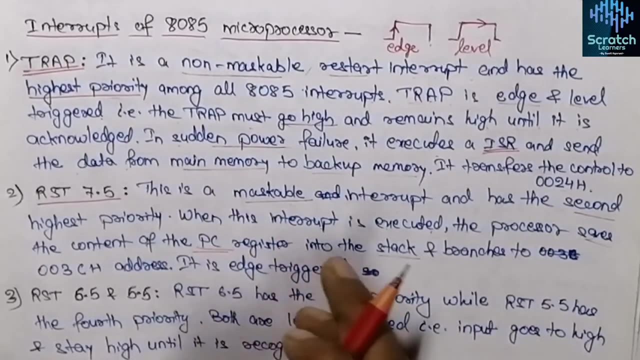 interrupt is executed, the processor saves the content of the pc register, that is, the program counter register, into the stack and branches to the 003c hex address. so as this is a maskable interrupt, it can be disabled easily and whenever such scenario is executed, that means whenever. 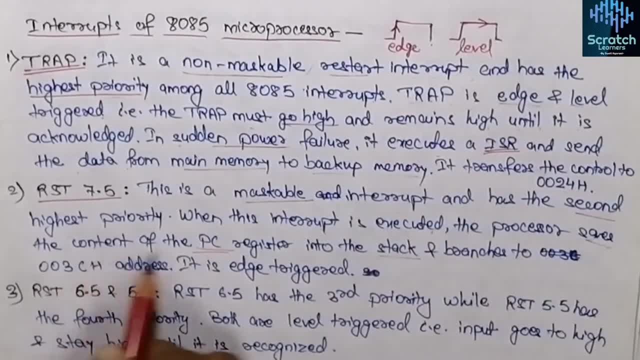 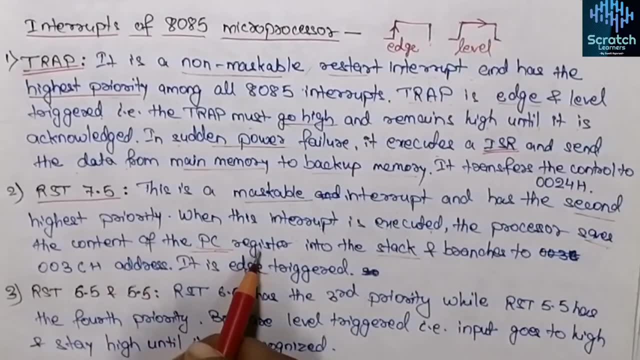 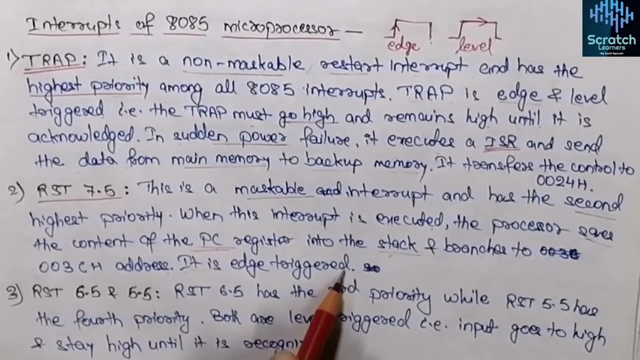 this interrupt is executed, the processor saves the content of the pc register. that means whatever work was being executed by the microprocessor, that is being saved into the stack and then the microprocessor branches to this address. so, as it is edge triggered, that means the input will go high and there is no need to. 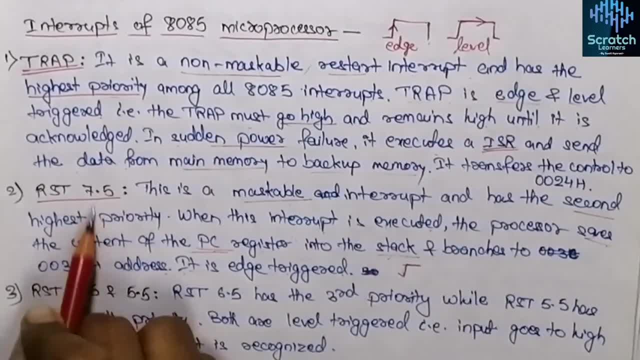 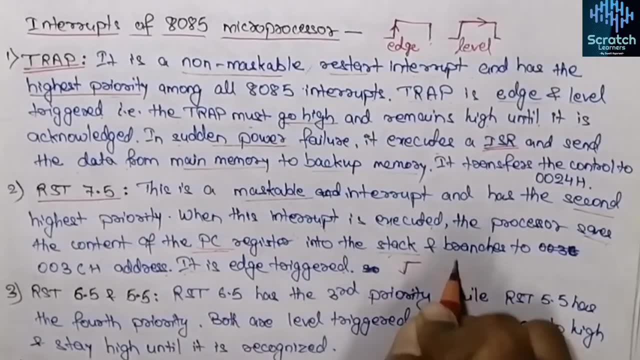 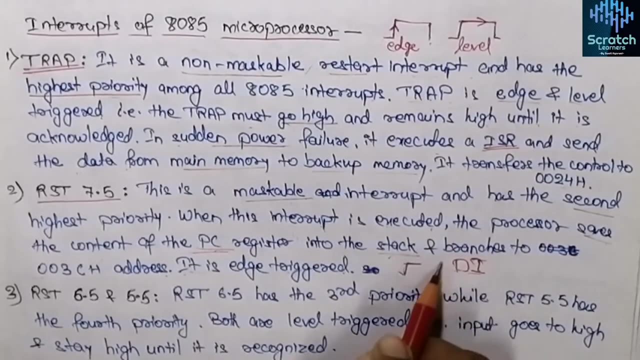 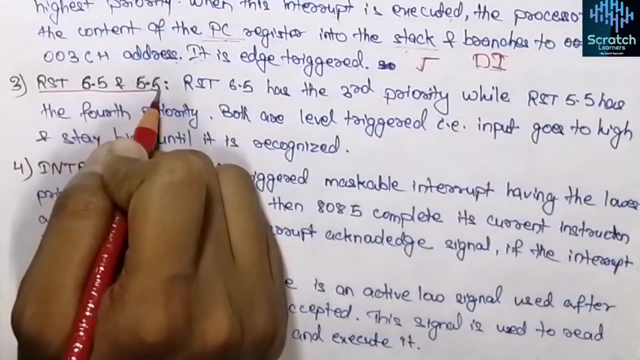 maintain the high state. and this rst 7.5 interrupt can also be masked by resetting the microprocessor or by resetting the di instruction. di instruction means disable, interrupt instruction. so by resetting the di rht 7.5 can be masked or disabled. now we have the rht 6.5 and 5.5. so the rht 6.5 has the 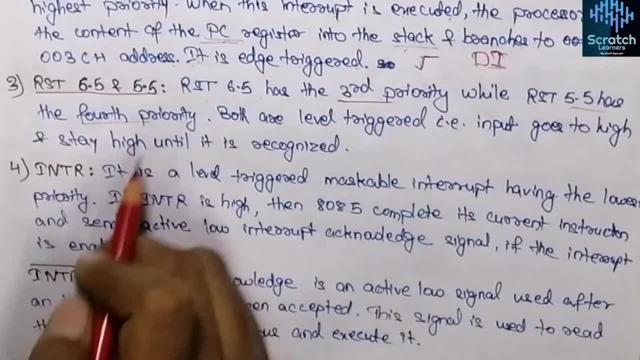 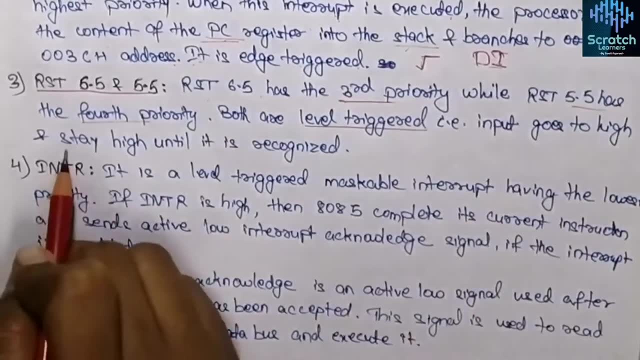 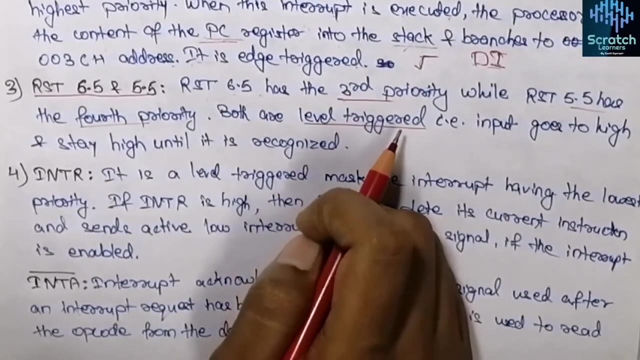 third priority, while rht 5.5 has the fourth priority, and both of these instructions are level triggered. that means the input goes to high and stays high until it is recognized. okay, we have just seen level triggering in case of trap, and these interrupts are also maskable interrupts. 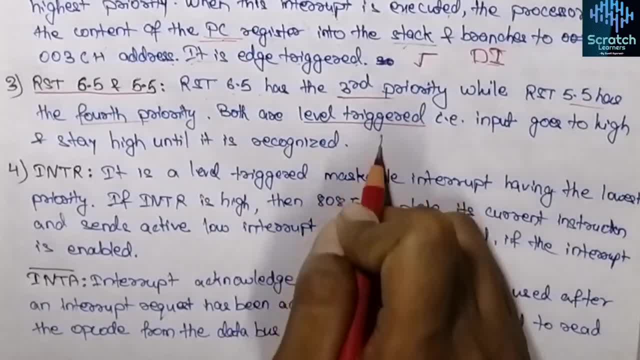 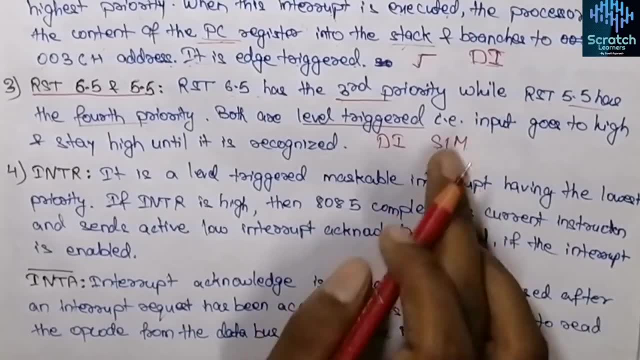 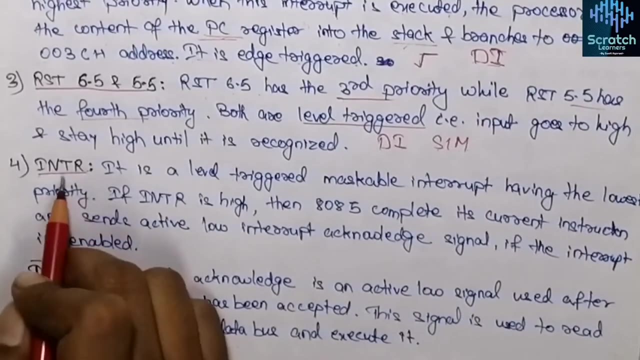 right. so these interrupts can be masked by using di, that means disable interrupt, and seam instruction, that means set interrupt mask, and it can also be masked by resetting the microprocessor. now the last one is the i interrupt r. so this is interrupt request. that means this is a level triggered maskable interrupt having the. 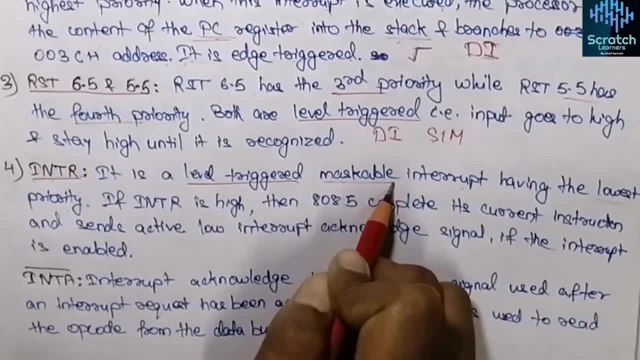 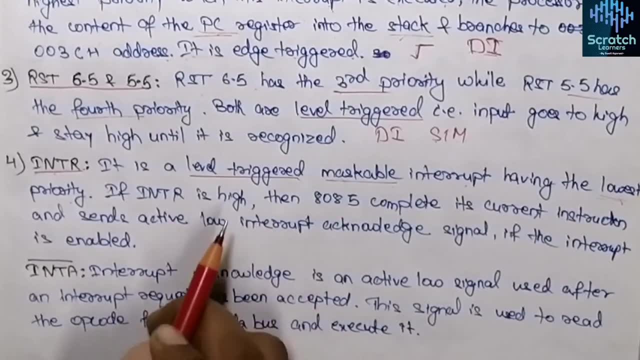 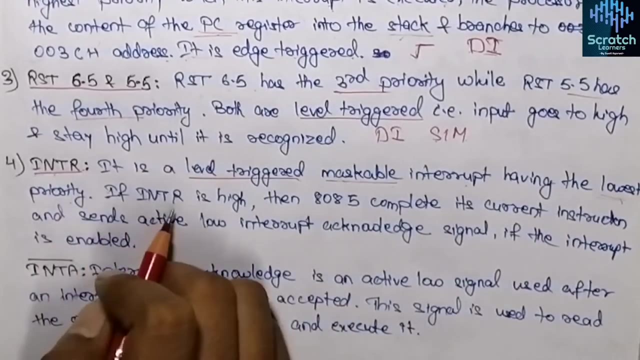 lowest priority. so this is easily maskable, as it is having the lowest priority among all the 8085 interrupts. so now how does microprocessor branches to an interrupt request? so in the beginning the 8085 checks the status of the intr signal during execution of each instruction.